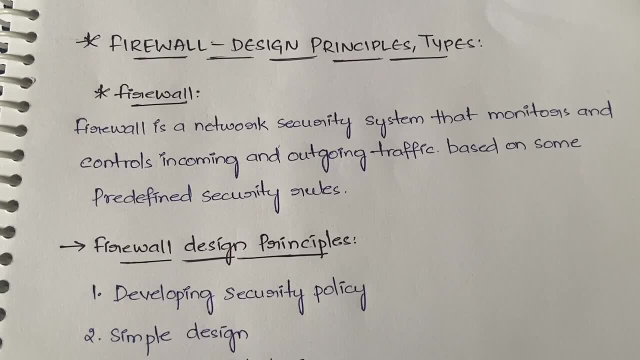 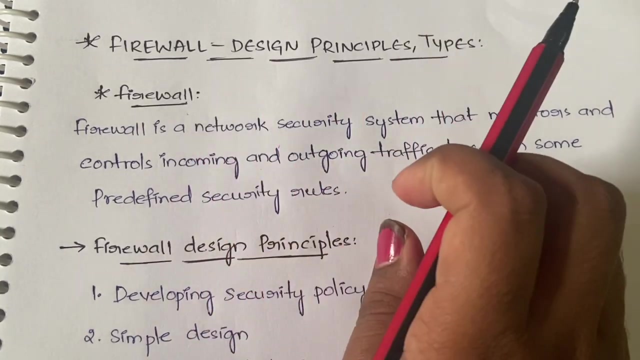 Hello everyone, welcome back to my YouTube channel, Trouble Free. In today's video I'm going to explain you about firewall, the design principles of firewall and, along with that, also the types of firewalls. also I'll be explaining you, Okay. so if types of firewalls is becoming a longer video, I'll be explaining it in the next part. Otherwise, in this video itself I'll cover, Okay. so first, first of all, basically what a firewall is. it is a network security system that will monitor and control the 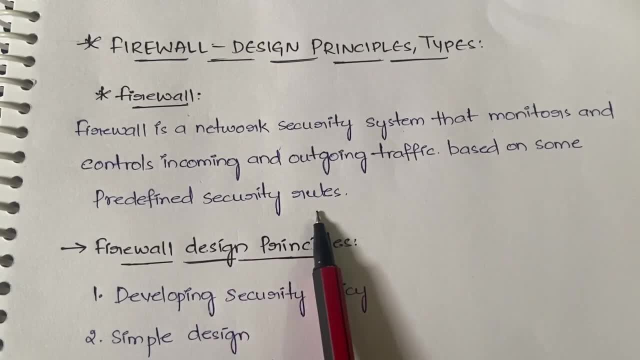 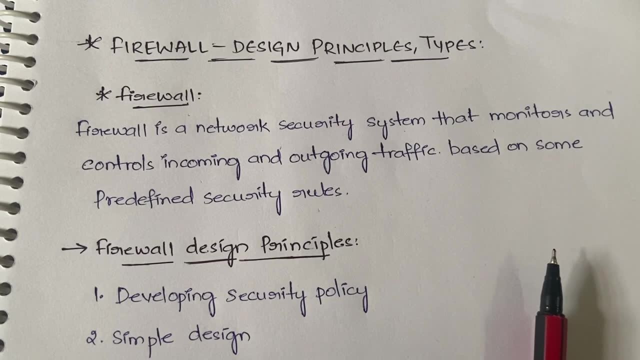 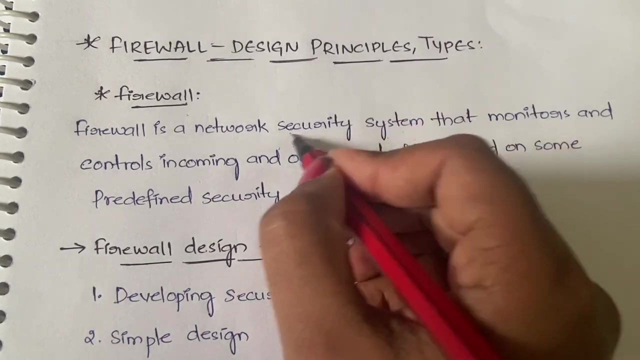 incoming and outgoing traffic based on some predefined security rules. Simple, don't get confused. It will simply prevent unwanted data from entering into our system. So it will prevent unwanted data, that is, the data which is causing harm to our system. it will avoid those kind of data. Got it? It is a network security system. It is basically used for security that will monitor, monitoring, innocence, observing and 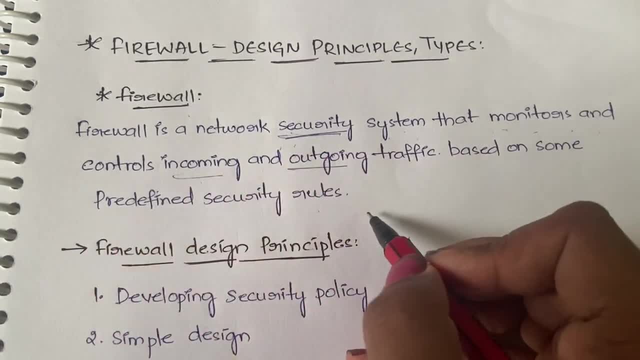 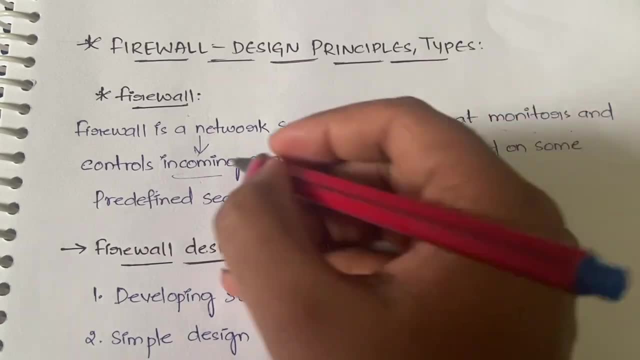 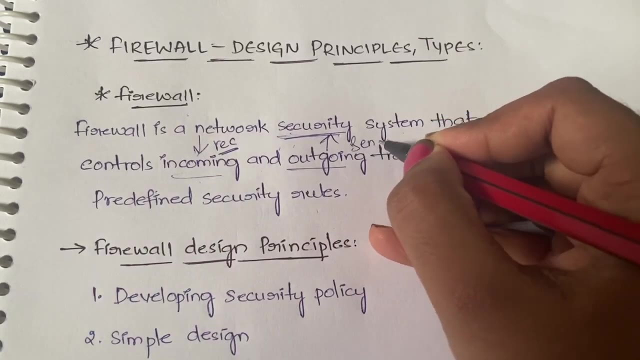 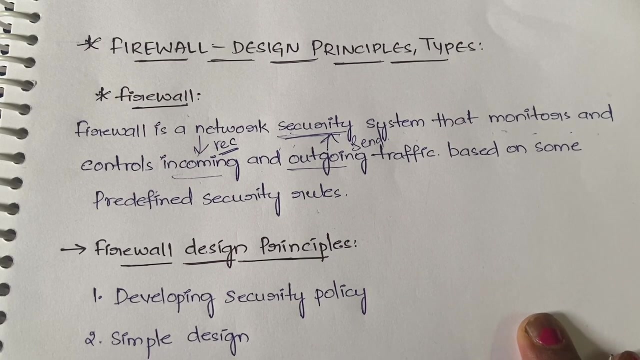 also, it will control the incoming and outgoing traffic. incoming traffic in the sense what is coming into our system. outgoing traffic in the sense what is going outside of our system, that is, the messages. incoming innocence, the messages which we are receiving. outgoing innocence, the messages which we are sending. okay, it will monitor both incoming and outgoing traffic based on some predefined security rules, Got it? So this is about firewall And not only monitoring. 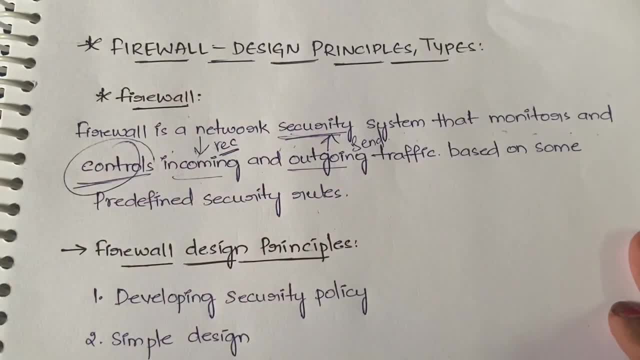 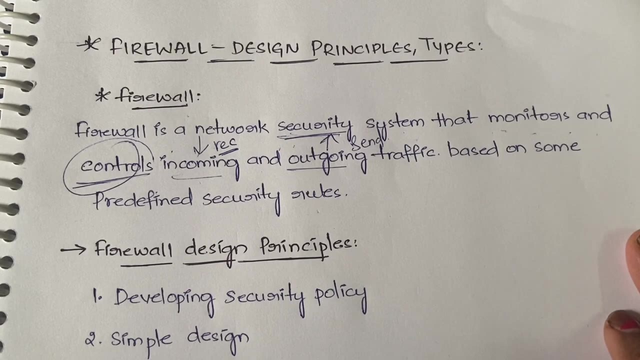 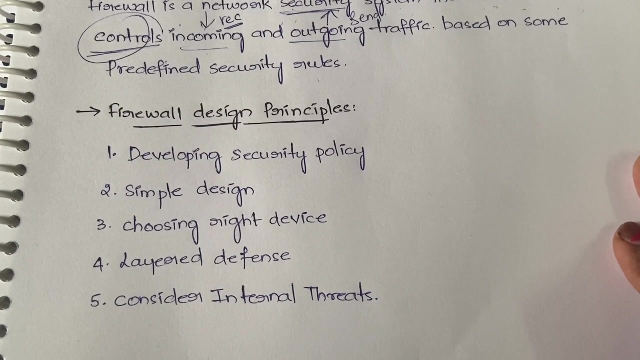 it will also do controlling. controlling in the sense if in case, if it identifies any unauthorized data or any harmful data or any vulnerable data, in that case it will stop that data. it will not allow the data to enter into our system, Got it? This is about firewall. Now let us see what are the design principles of firewall. What do you mean by firewall? design principles, Simple: when you're designing a firewall or when you're developing a firewall, when you're designing 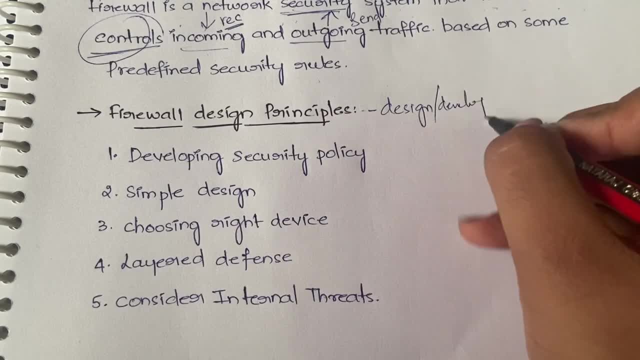 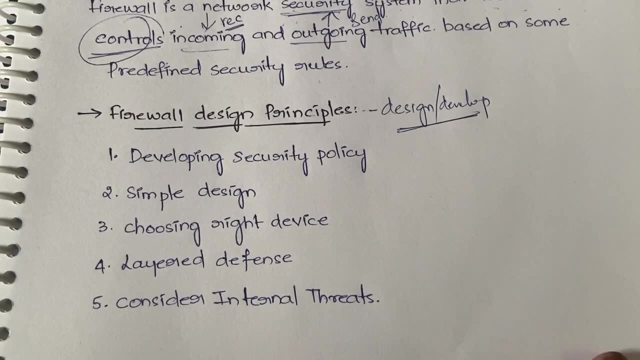 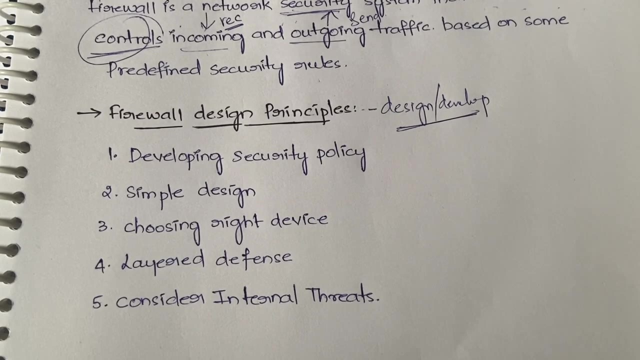 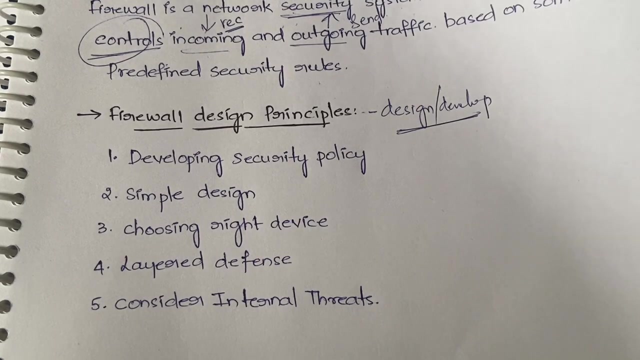 or when you're developing a firewall, you need to keep some things in your mind, right? Suppose if you're, if you have to, if you're writing an answer. suppose the question is like: what is firewall And what are the design principles of firewall And what are the types of firewall? If this is a question, then what all you have to keep in your mind? you need to answer what a firewall is, you have to answer what are the design principles of firewall and you have to answer what are the types of firewall. the same way, when you're when 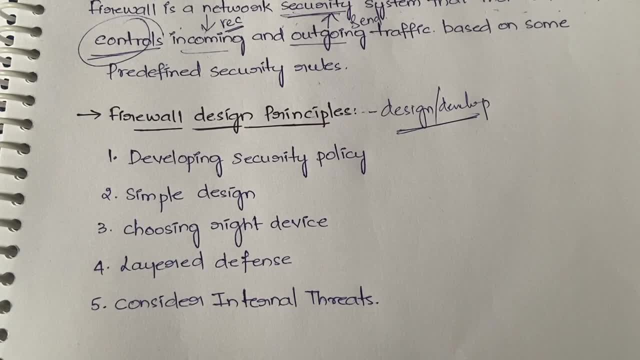 you're doing something, you will be keeping in mind something like: okay, all these purposes have to be done. so the same way, when you're designing a firewall, you need to keep some things in your mind. okay, what are those? let us see. first, is developing a security policy, so developing a. 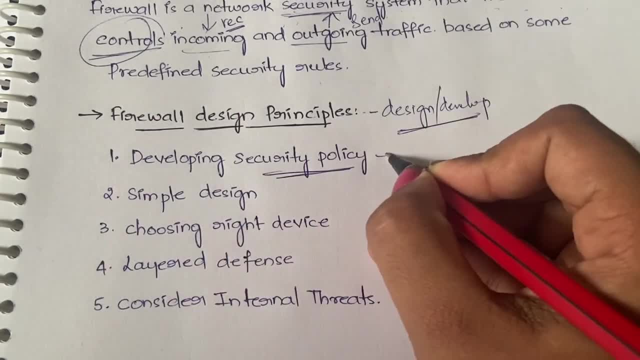 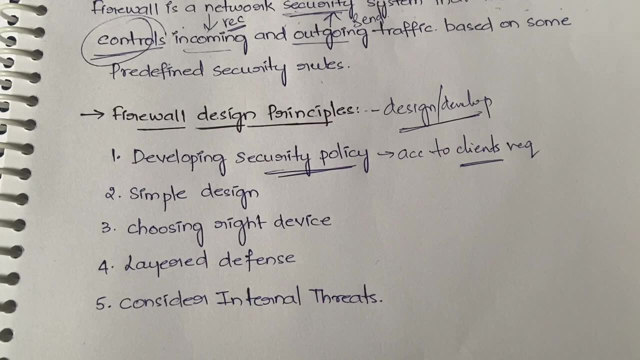 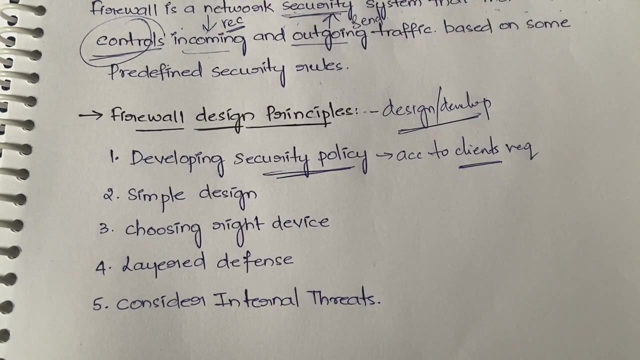 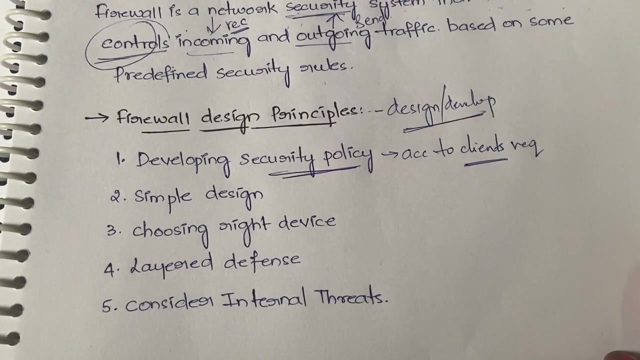 security policy is nothing, but we should develop a security policy according to the client's requirements. okay, so who is your client, to whom you are working? they will be your client. okay, so a security policy has to be developed according to the client limit- sorry, requirement- and also according to the type of traffic of the client. suppose if a client is a college website. 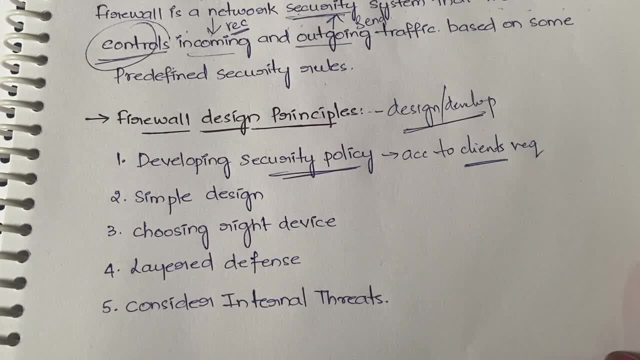 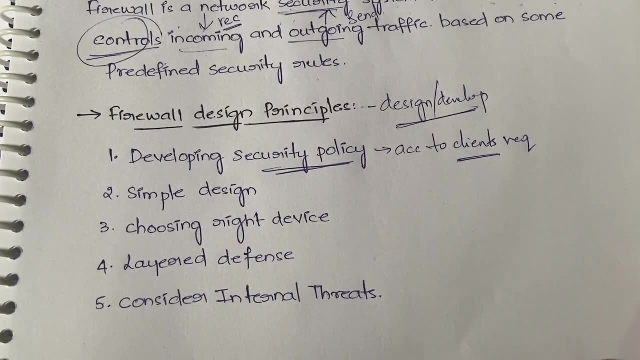 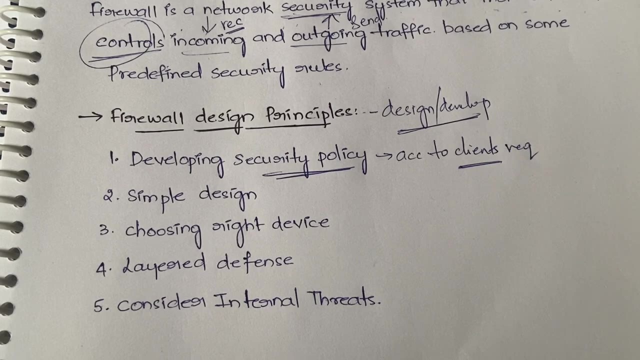 then what will be the traffic? college students or college faculty- those kind of people will be the client also. i mean the like. those kind of people will be visiting the website, right? if suppose if it is a railway booking system, then different kinds of people will be visiting that site. so, based on the traffic which is coming to that site, that is based. 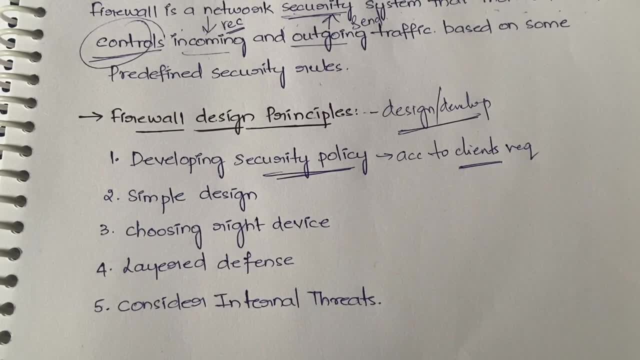 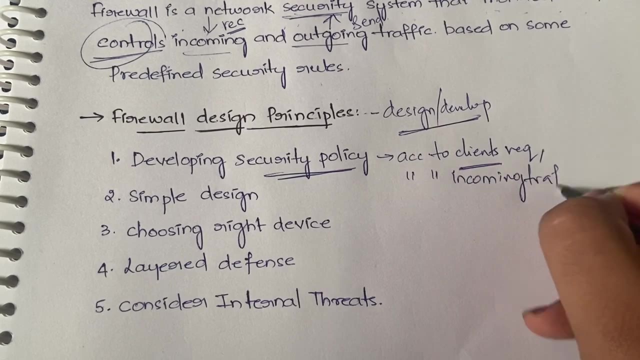 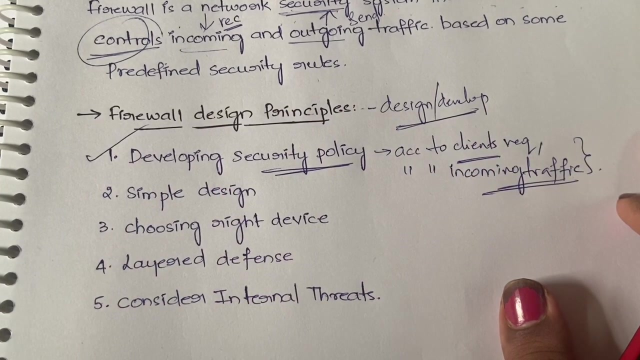 on the types of people who are visiting that site. the security policy has to be developed. so the security policy has to be developed according to the client's requirements and also according to the incoming traffic. okay, by keeping these two things in mind, you need to develop the security policy. next, simple design: 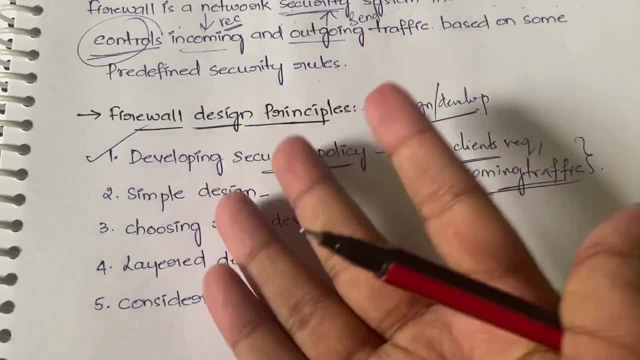 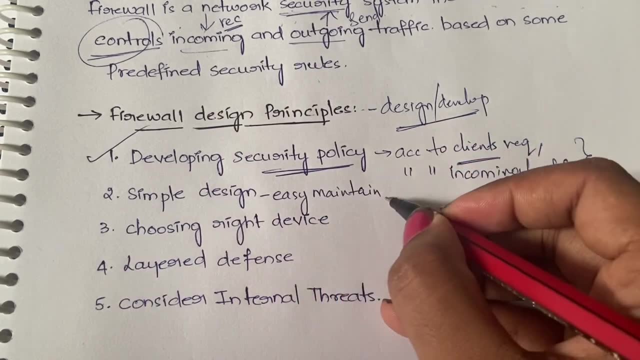 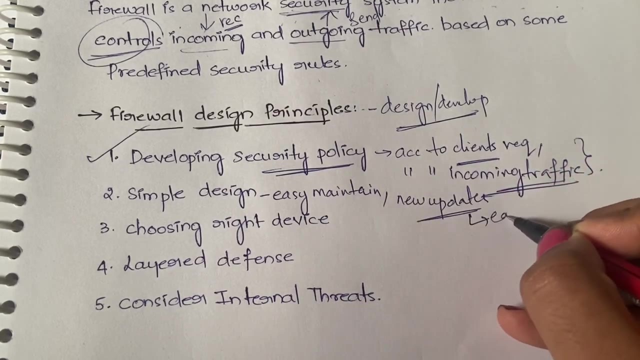 why simple design? simple design: if you are having a simple design, two advantages you will have: it will be easy to maintain. easy maintenance will be there along with that. if there are any new updates. okay, if there are any new updates, those new updates can be easily done. if the system is very hard, if the design is very complicated, then it 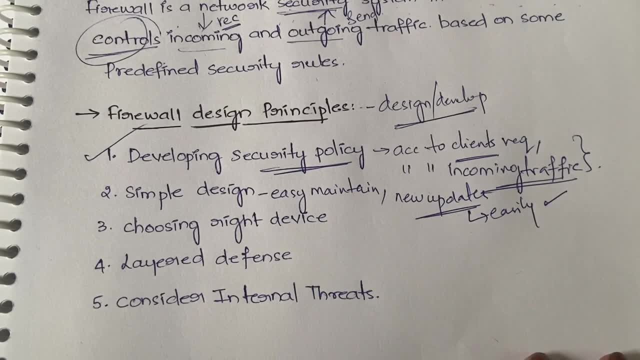 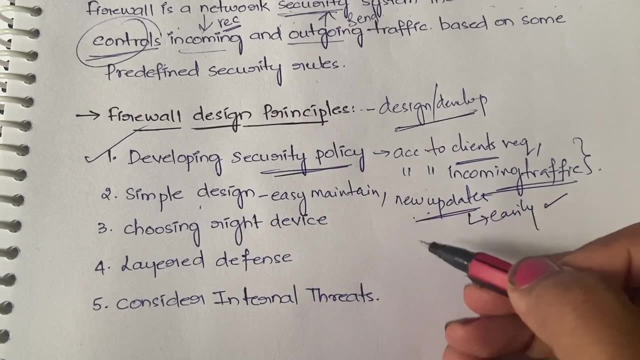 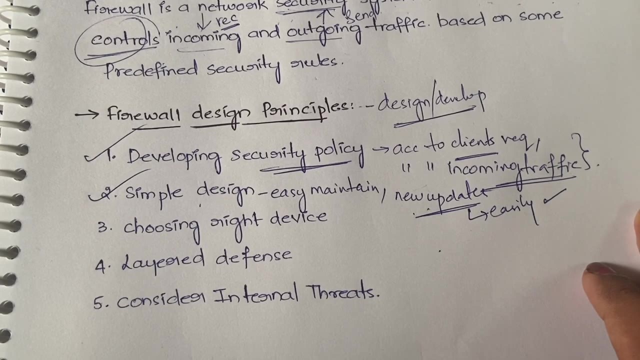 is very hard to understand the system and do some updates on the system. right? so if the system is, if the design is simple, you can easily maintenance, maintain and, along with that, if there are any new updates, you can easily update your system. okay, choosing the right device. so, which is nothing, but when 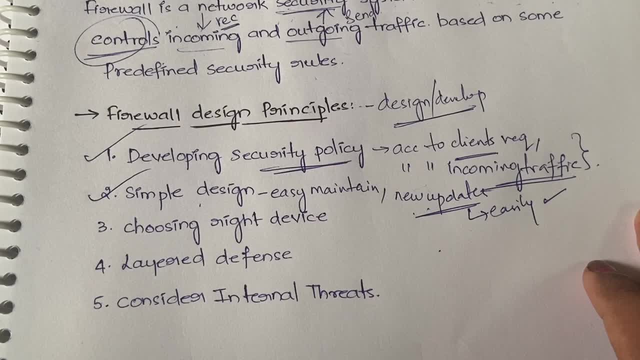 you are designing a firewall. suppose you are designing a firewall on your system, on your laptop, then it has to be a secured system. it has to be a well-defined system. you should not use outdated system. so when you are designing a firewall, the device on which you are defined 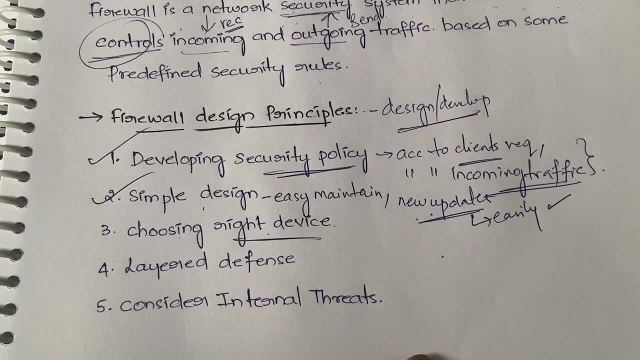 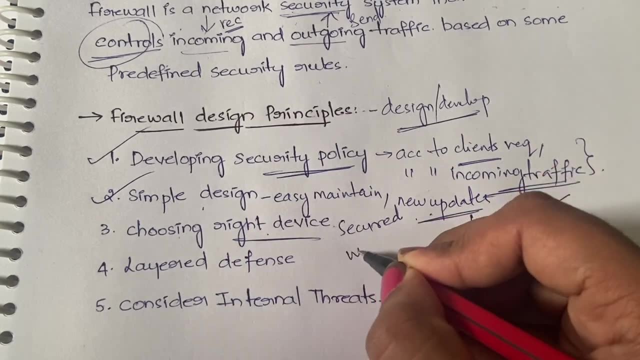 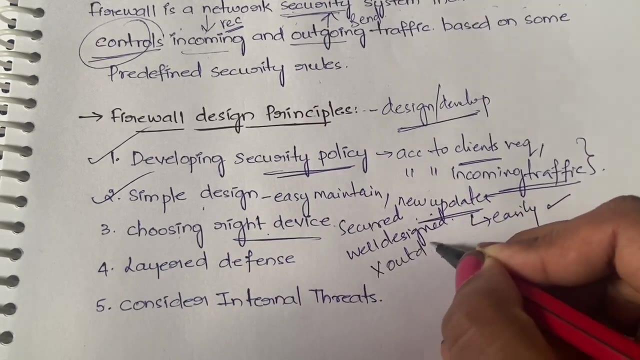 sorry, sorry. the device on which you are designing your firewall has to be fully secured. okay, it has to be fully secured, and the design should be. it has to be well designed and, along with that, also, you have to not use outdated systems, got it? so when you are designing a firewall, 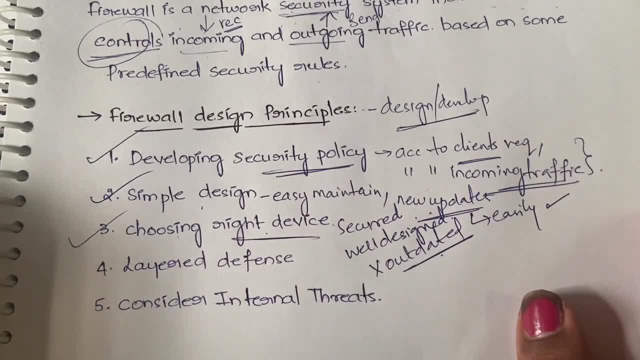 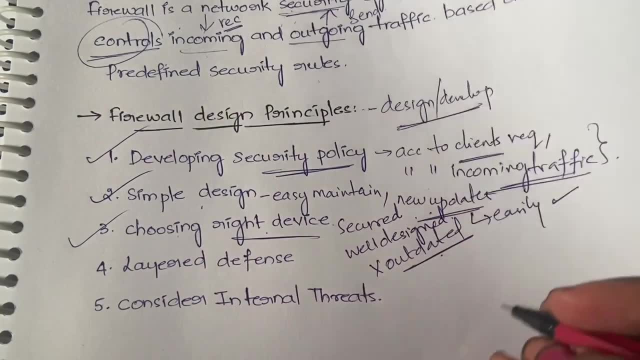 you need to keep all these things in your mind. next comes the layer defines. so what do you mean by layer defense? layer defense is nothing, but the design should be multi-layered, because suppose you are designing the firewall, that has to be, that has to have multi-layer. 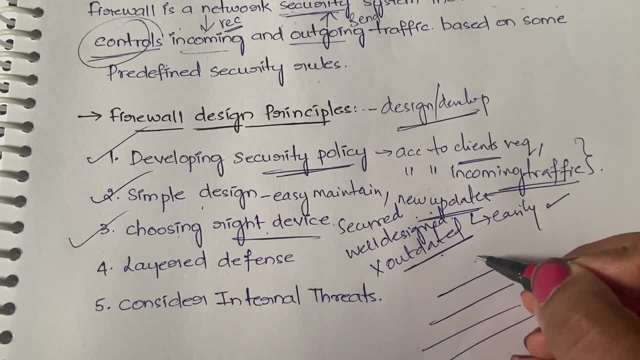 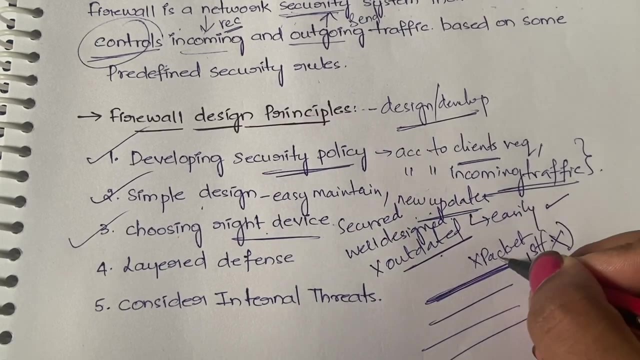 security, if at all, if some, you know some harmful packet is coming, harmful data packet is coming from this layer, it so in this layer, first level of checking will be done. so, if at all, by chance, if the, if it is missed, if the protection is missed and this packet came to this layer, 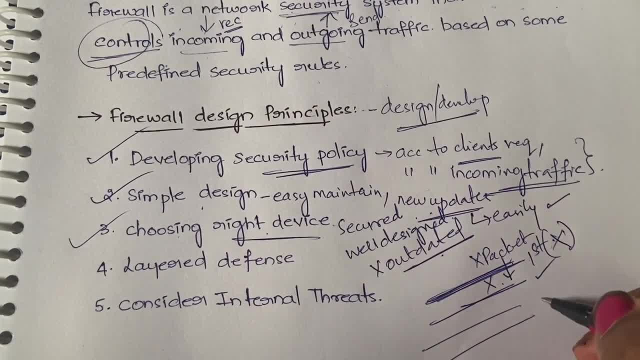 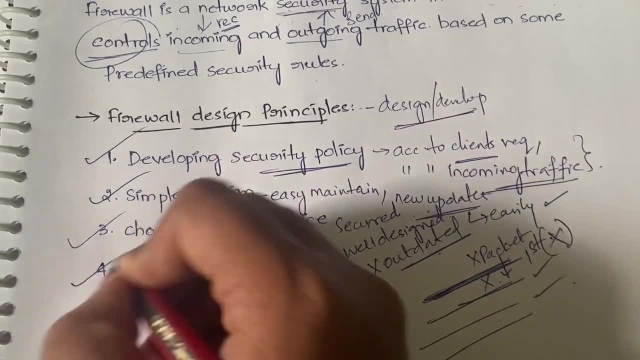 also at his. it has to detect in this layer, if not at least in this. So it has to be multi-layered so that at different, different labels it can check. okay, and also you need to consider the internal threats. that is what can happen through the through. 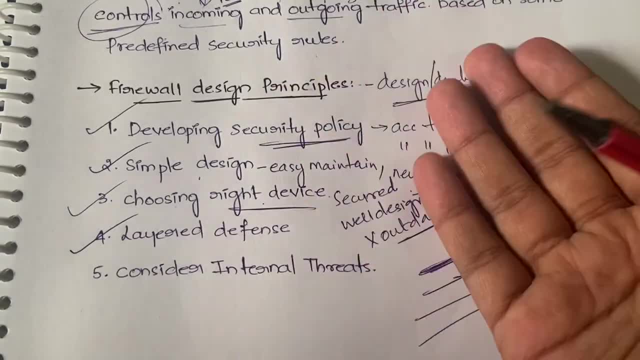 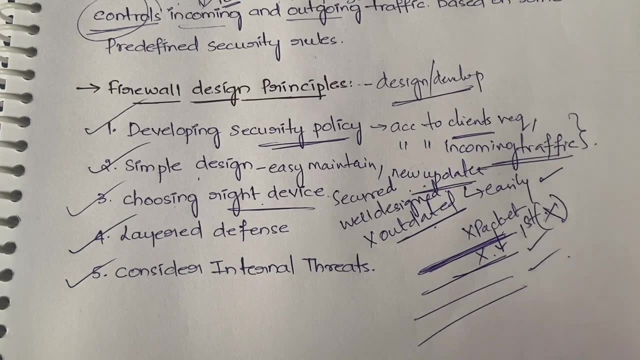 inside of the computer, from inside of the device, what kind of different threats can arise? those also you should keep in your mind while you are designing a firewall. okay, so after this, I think we have types of firewalls. yes, so I'm stopping this video now in the 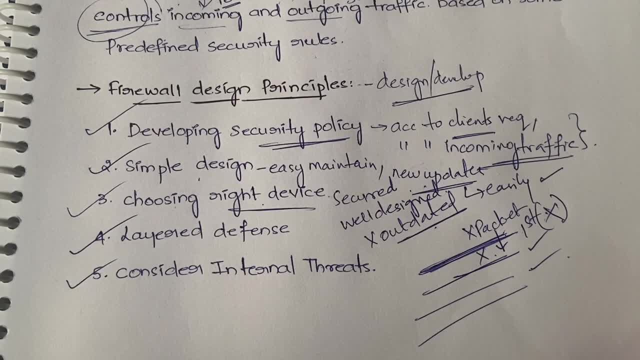 next video. Let's talk again about the types of firewalls. we have three types, okay, so we have packet and we have application level and we have circuit level. okay, these three things I'll explain in the next video. thanks for watching the video till the end. let's meet up in the